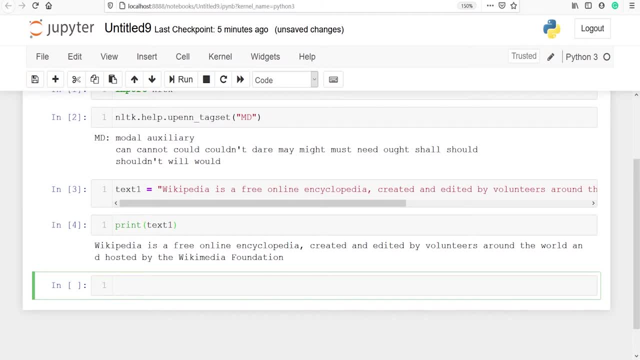 Let's tokenize, That is, we will take out words from the sentence saved in the variable text1.. I'll make one variable words1, and now I will call our variable text1.. We will tokenize, That is, we will break the sentence into words and we will extract words from this sentence. 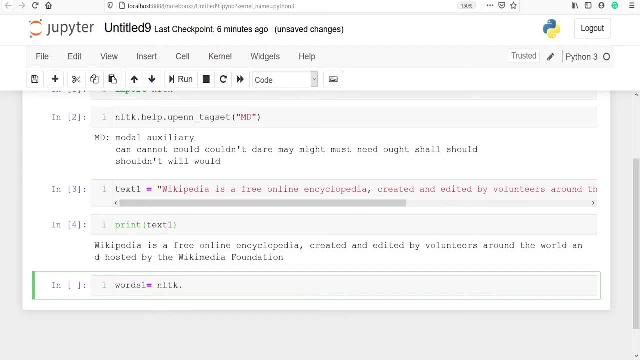 from nltk. I'll call the method: word underscore text1.. This will convert those words in to text. We will call it text2.. Because text2 is an integer, the method is initialized. You can call this method: word underscore text1.. score tokenize and then I will pass our variable text one. let's execute our code. 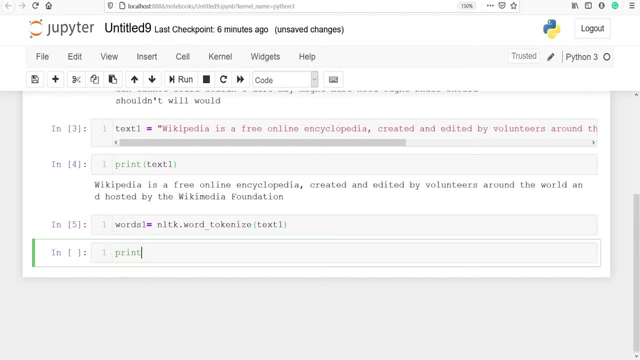 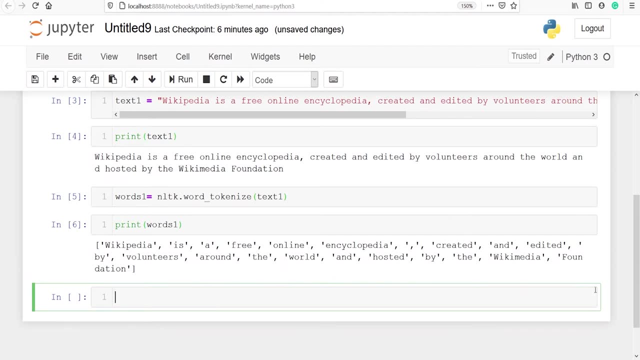 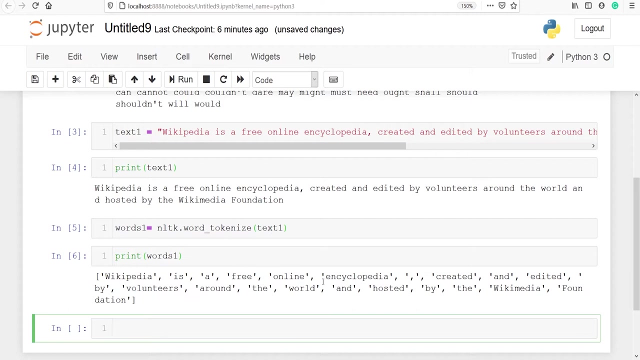 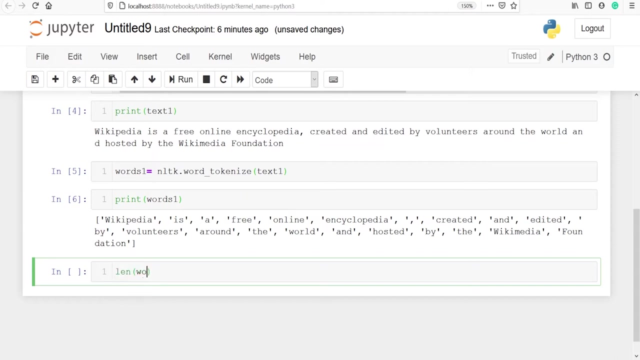 let's print our variable words. one in the output. you can see that we have tokenize our sentence in variable text. one, and these are the words: Wikipedia is AF, free, online, and so on. we can also look at the length of these words. I type length and then words. one in the output you can see that we got 21 because there 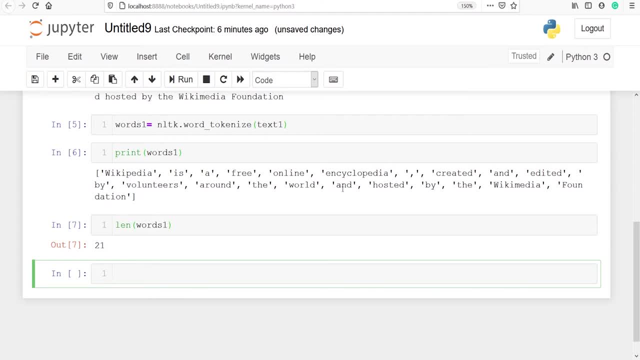 are total 21 words in this variable words one. now we will do the parts of speech tagging from NLTK. I will call POS underscore tag. you can also look at the size of the text and then you can also look at the. and then I will pass our variable words, one in which we have saved our tokenized 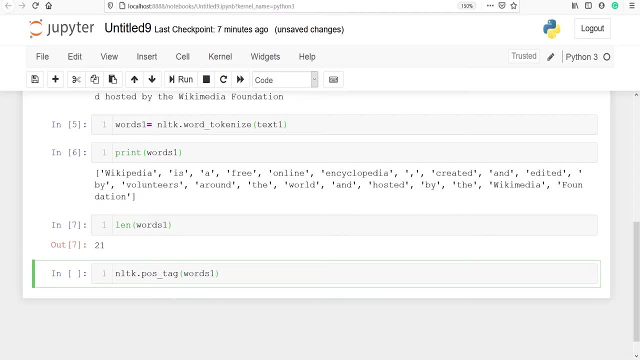 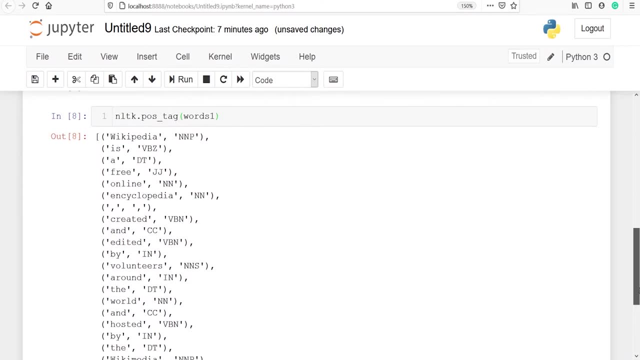 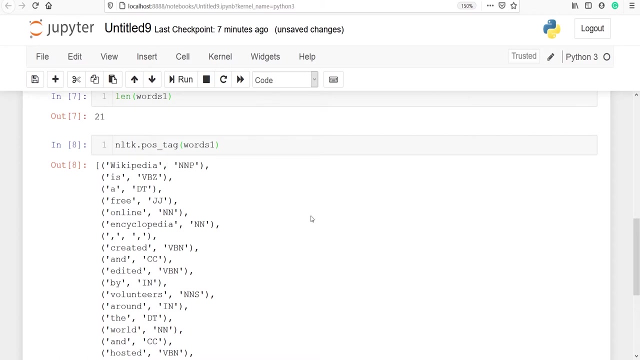 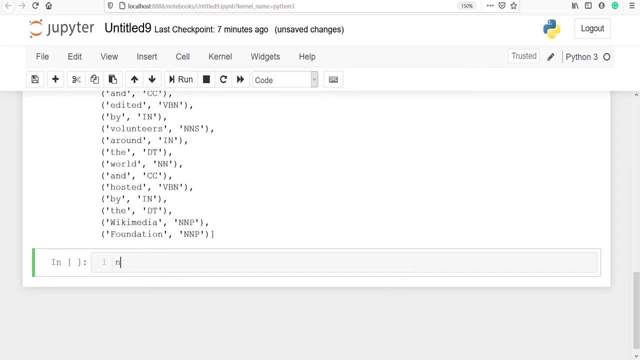 words, words, one. in the output you can see that we have done parts of speech tagging and all these are verbs and all we need to know the full form of this. and to get the full form we have one function here from NLTK: dot help, dot, brown text set. let's execute our code and here you will find the full form of. 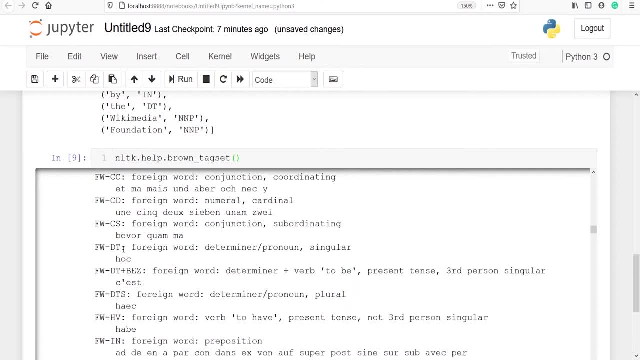 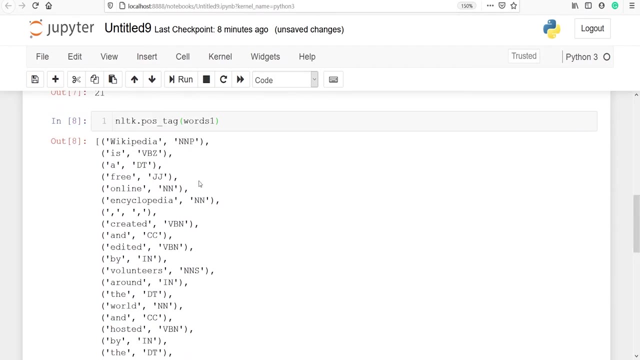 words here, for example, here DT. so you will see, here DT is determiner or pronoun. then we have CD, it is numeral cardinal and here you will see that we have what, some short forms here, such as NNP, VBZ, DT, JJ, and to get the full form of a particular 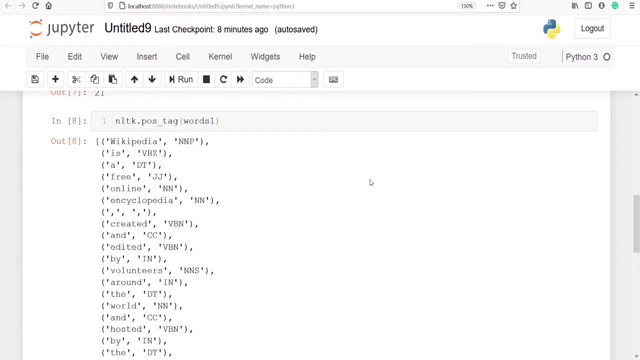 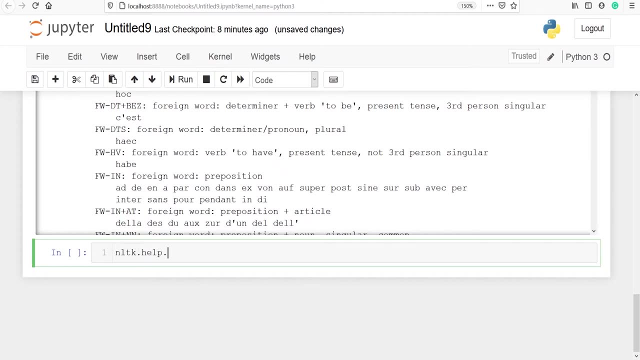 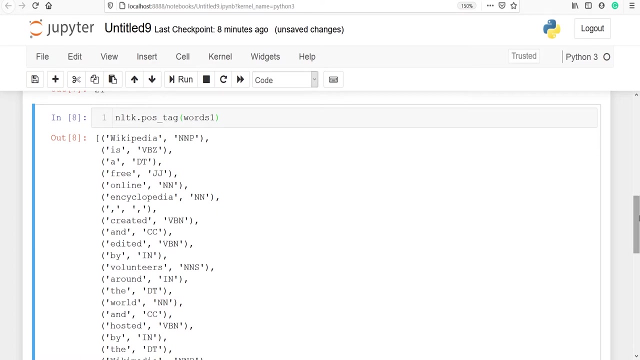 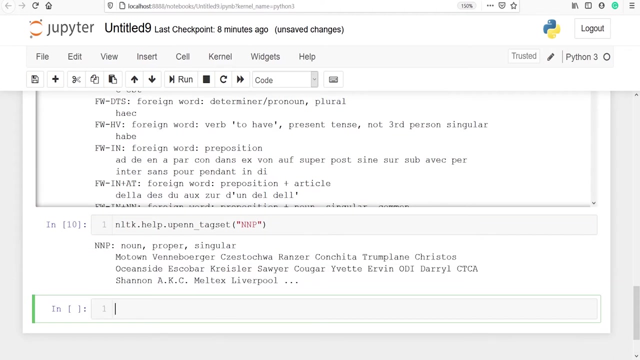 this short form, particular POS. there is one more method, so I'll type NL, TK, dot-help, dot, UP, ENL. and now we want to know the full form of this NNP. I'll copy this NNP from here. I'll paste it here in double quotes. let's execute our code. NNP stands for noun, proper singular. similarly, 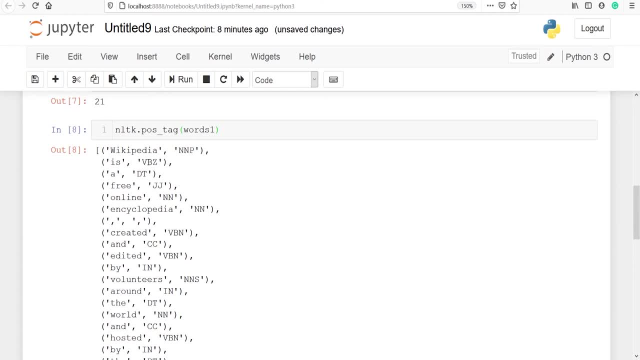 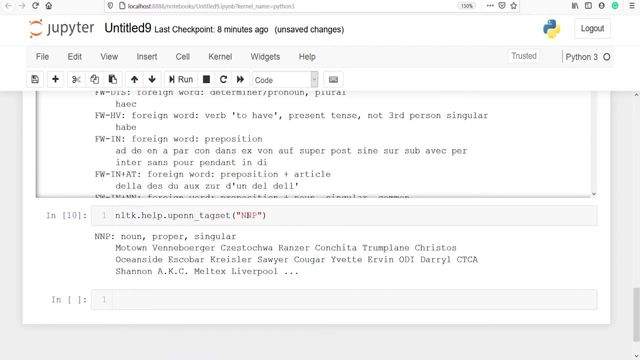 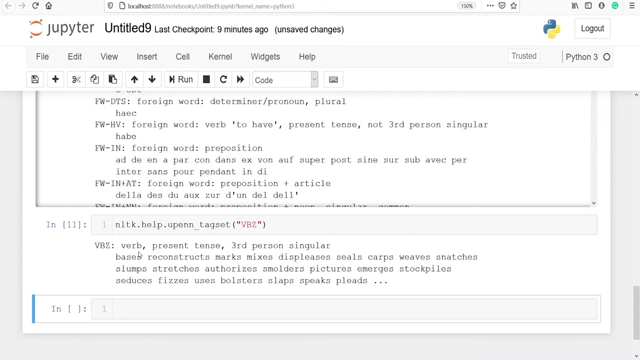 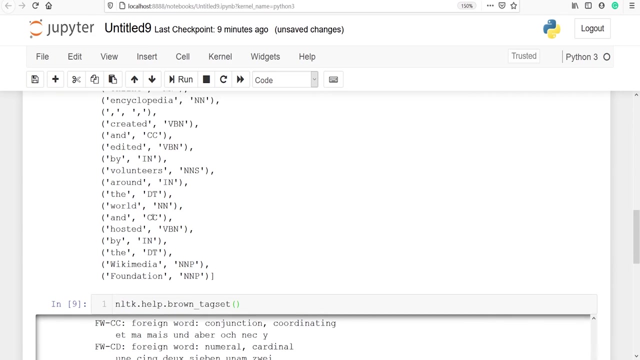 we can look at some other codes, for example VBZ. I'll copy this from here. I'll paste it here. let's execute our code. VBZ stands for verb present tense third person singular. we can also look at some other codes. let's look at this CC. let's paste it here in double quotes. 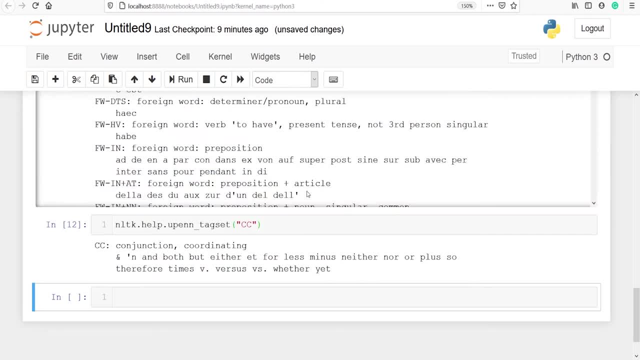 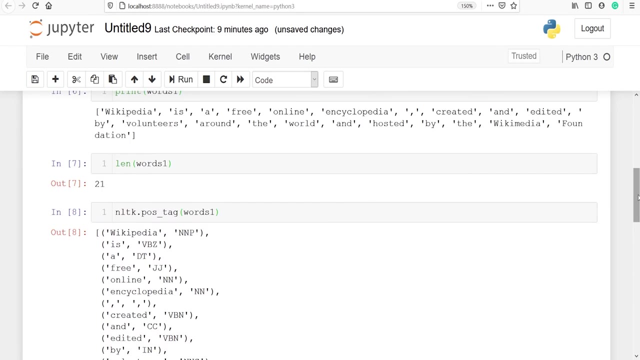 let's execute our code and here in the output we will see that CC stands for conjunction, co-ordinating. this is how you can find the full form of each and every POS and to do the parts of speech tagging. first we have to convert our sentence into words and we 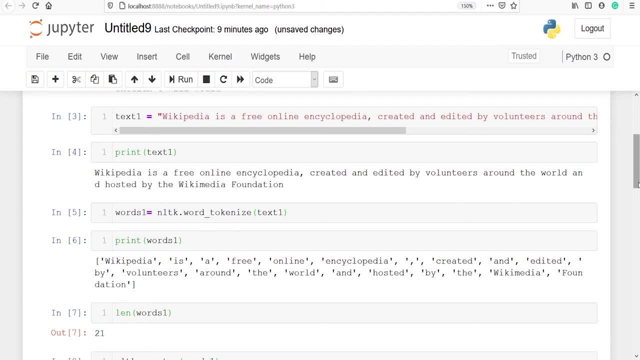 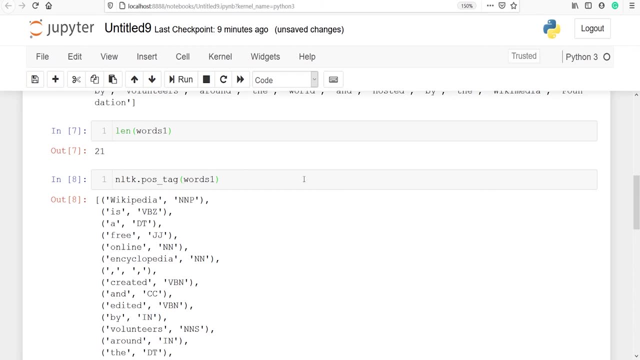 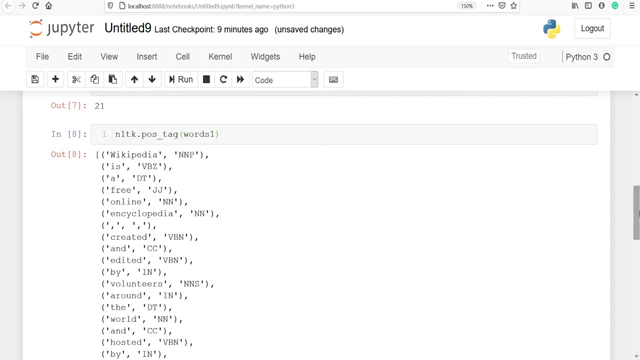 can do that using word underscore tokenize, and once we have break down our sentence into then we can call our part of speech, tagging on our words, and once we do that we will get all the parts of speech for each and every word and to get the full. 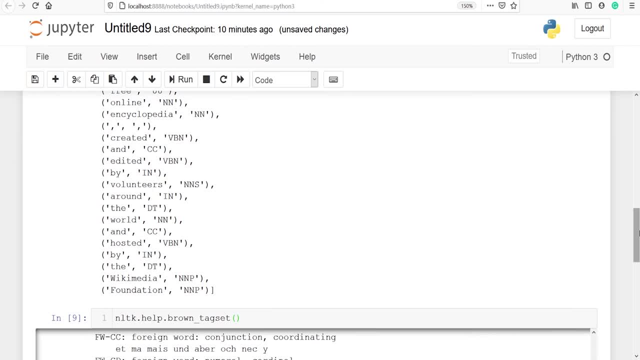 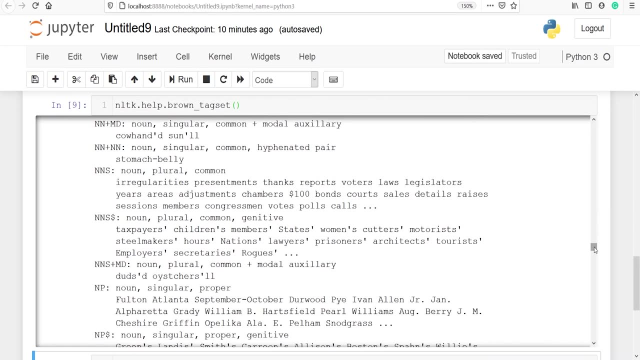 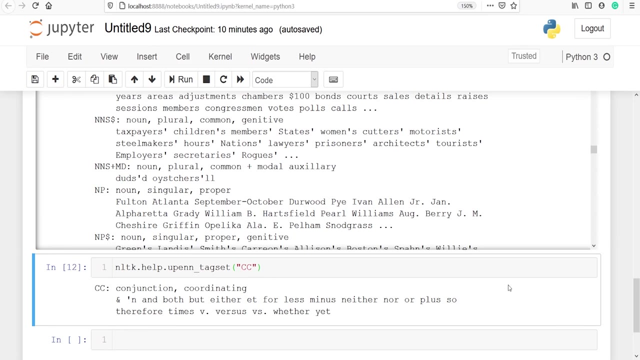 form of all these POS parts of speech. we can use the help method. using this method, you will get all the full form here and if you want a particular full form, you can use this another help method and you can put the POS here and get the full form of that. if you liked my video, please subscribe to my channel. thank you for watching.